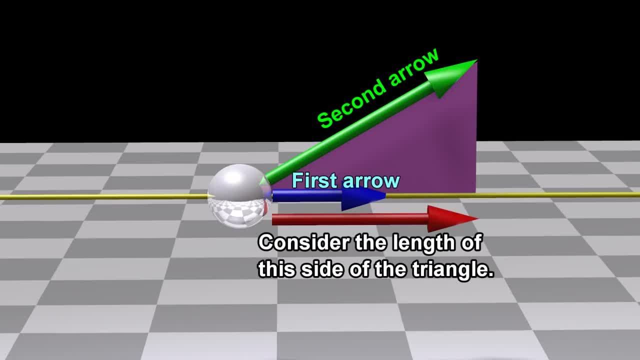 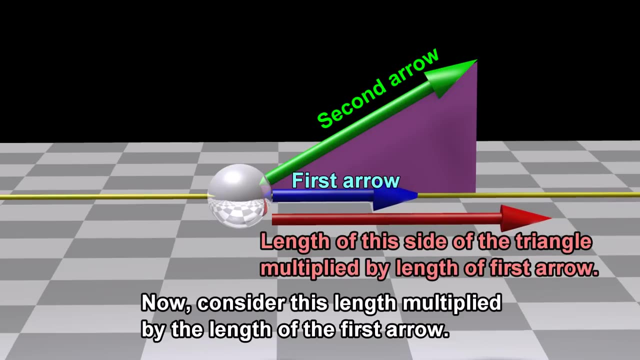 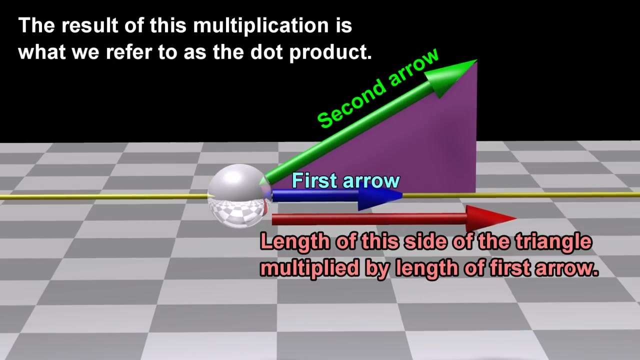 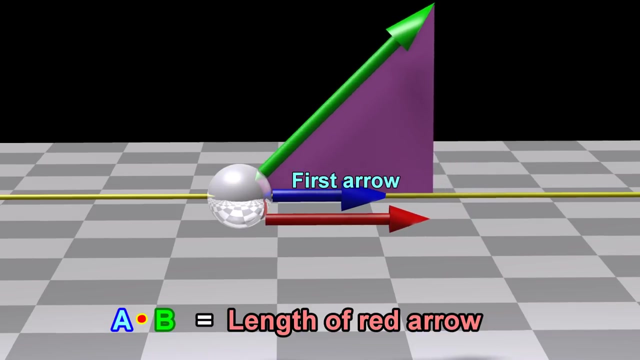 Consider the length of this side of the triangle. Now consider this length multiplied by the length of the first arrow. The result of this multiplication is what we refer to as the dot product. If the first arrow and the red arrow are pointed in opposite directions, then the dot product is negative. 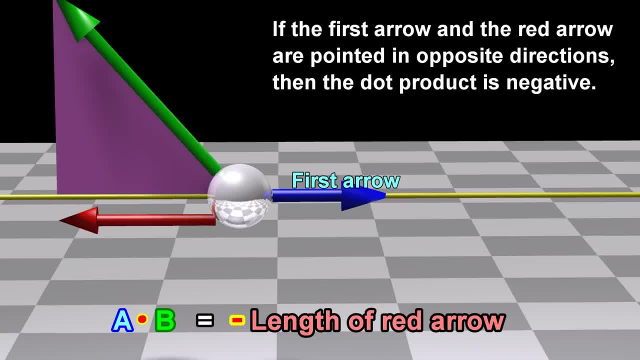 If the first arrow and the red arrow are pointed in opposite directions, then the dot product is negative. If the first arrow and the red arrow are pointed in opposite directions, then the dot product is negative. This means that the first arrow is the same as its dot product. 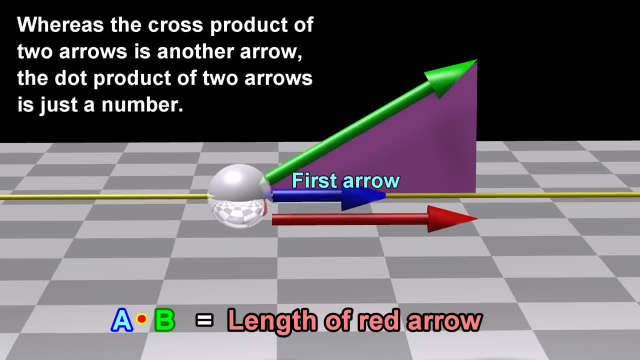 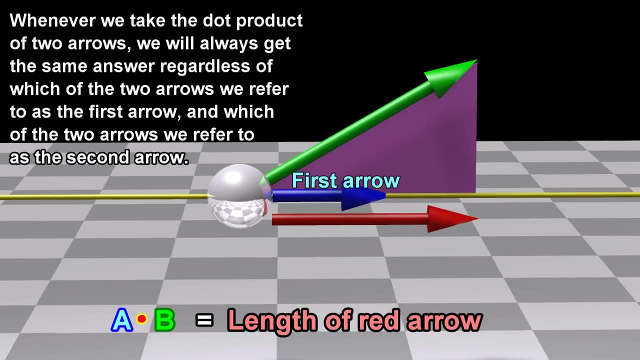 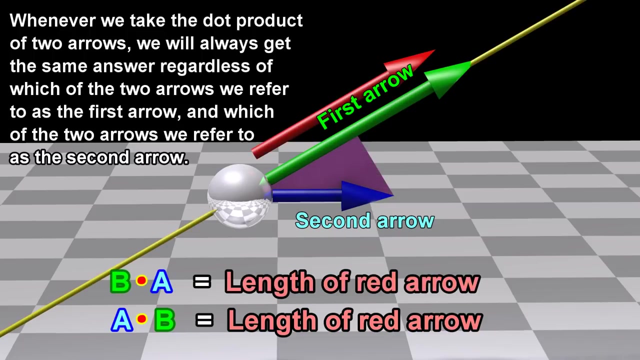 Whereas the cross product of two arrows is another arrow, the dot product of two arrows is just a number. Whenever we take the dot product of two arrows, answer regardless of which of the two arrows we refer to as the first arrow and which of the two arrows we refer to as the second arrow. 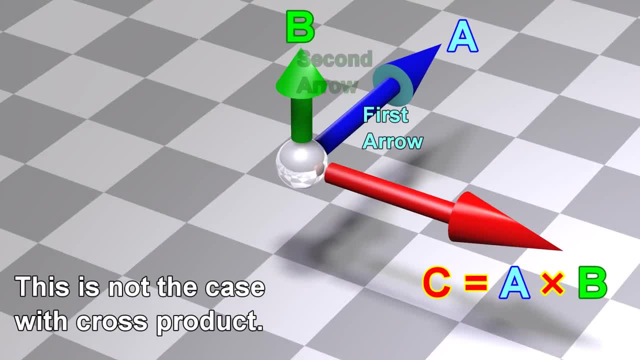 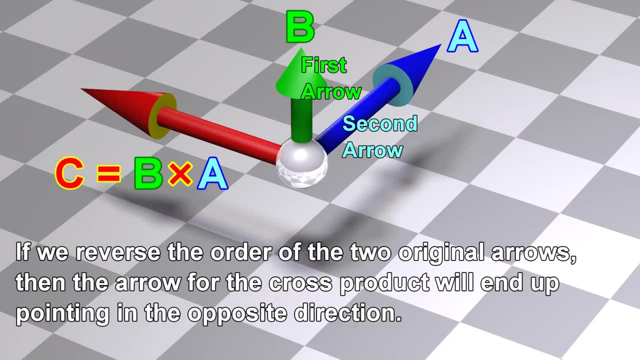 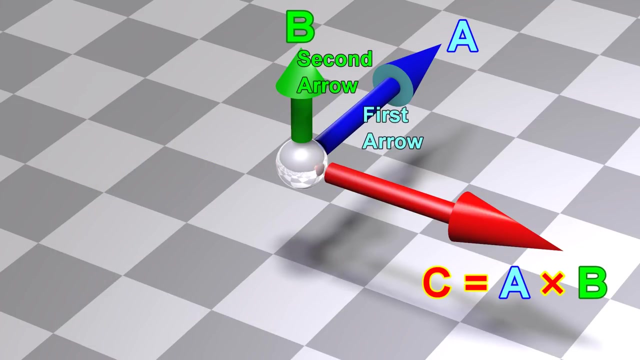 This is not the case with cross product. If we reverse the order of the two original arrows, then the arrow for the cross product will end up pointing in the opposite direction. There's a rule for using your right hand to remember the direction in which the 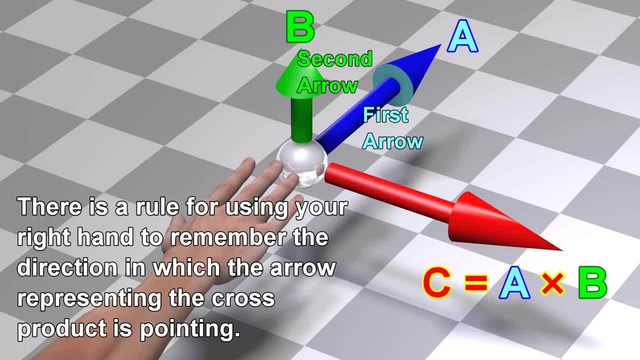 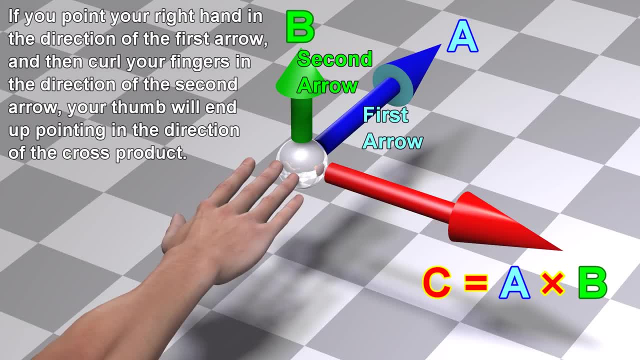 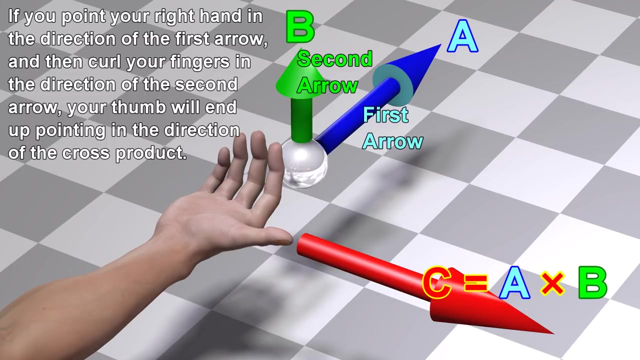 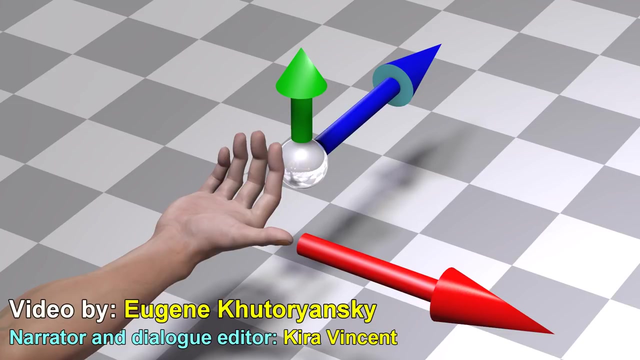 arrow representing the cross product is pointing. If you point your right hand in the direction of the first arrow and then curl your fingers in the direction of the second arrow, your thumb will end up pointing in the direction of the cross product. Much more information is available in the other videos on this channel and. 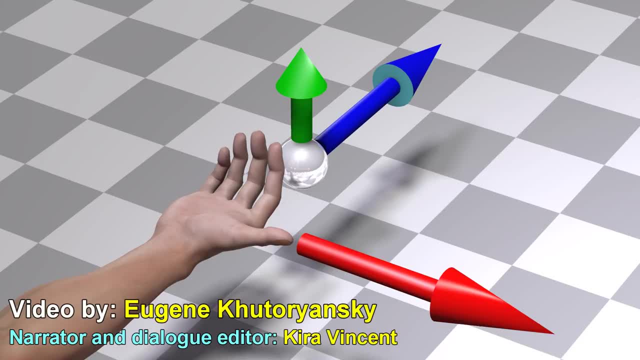 please subscribe for notifications when new videos are ready. Thanks for watching.